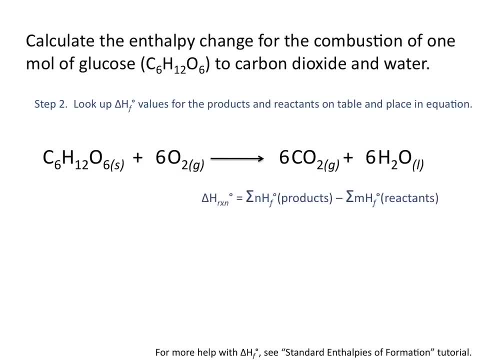 on the table and place them in our equation. Remember that the enthalpy of reaction is equal to the sum of the enthalpies of formation of the products times their respective coefficients, minus the enthalpies of formation of the reactants multiplied by their coefficients. Now in order. 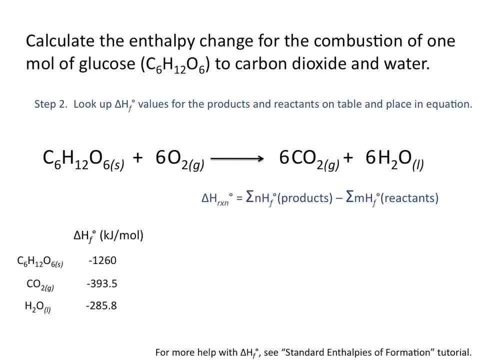 to do these problems, you would be given a table listing the enthalpies of formation of various different compounds, But in this example, to save space, I've listed only the values that we will need for this problem. The other thing that's important when doing these problems is to specify the state of 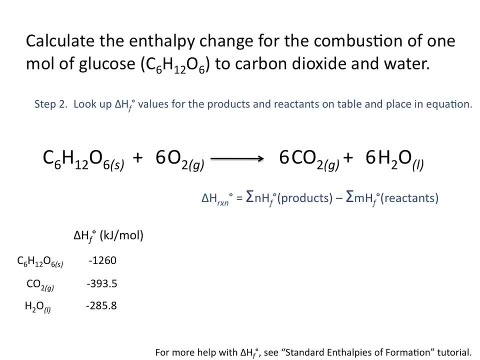 your reactants and products, because the enthalpy of formation values differ depending on the state of a compound. So, for example, the enthalpy of formation of liquid water is different than that of the enthalpy of formation of solid water or gaseous water. 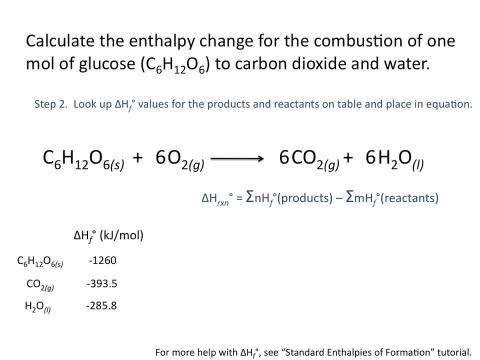 You'll also notice that in my enthalpy of formation values, O2 is not listed. This is because the element oxygen exists in the standard state as a gas, and so the enthalpy of formation value is zero, and this holds true for any element in its standard state. 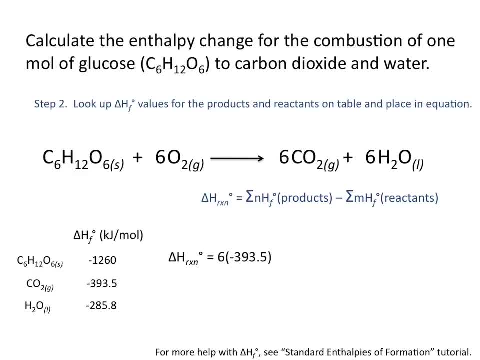 Now let's plug these values into our problem. First, we're looking at the sum of the enthalpy of formation values for the products, Starting with CO2, I can see that the enthalpy of formation value is negative: 393.5 kilojoules. 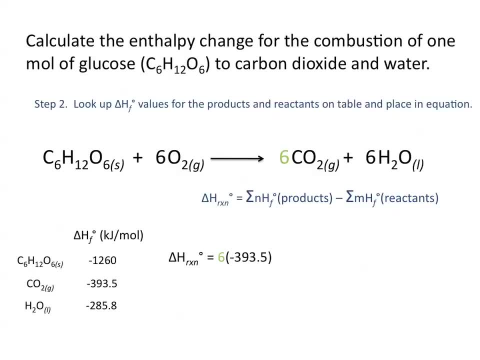 per mol, And I multiply this value by six because 6 is the coefficient in front of CO2 and our balanced chemical equation And because I used the coefficients in my balanced chemical equation. this is why it's particularly important to balance your equation correctly. 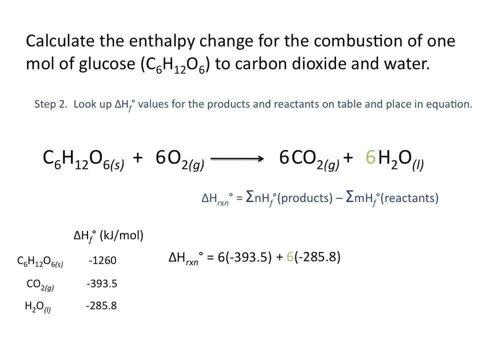 Also on my product side, I have water. so I take six, which is the coefficient in front of h2o, and multiply that by the enthalpy of formation value for water in its liquid form, which is negative. two hundred eighty five point eight kilojoules per mole. this is the 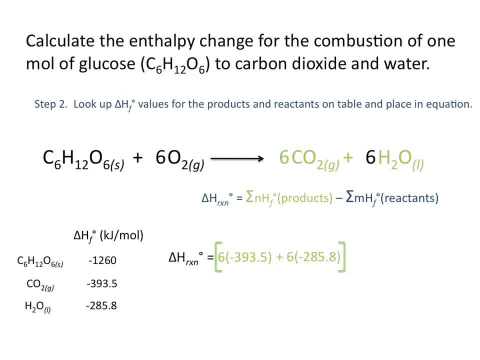 sum of the enthalpy of formation values for the products, multiplied by their respective coefficients. I then subtract the values for the reactants. I have one, glucose, so I take one multiplied by negative, 1260 kilojoules per mole, and then, remember I stated that the value of oxygen, because it's an element in its 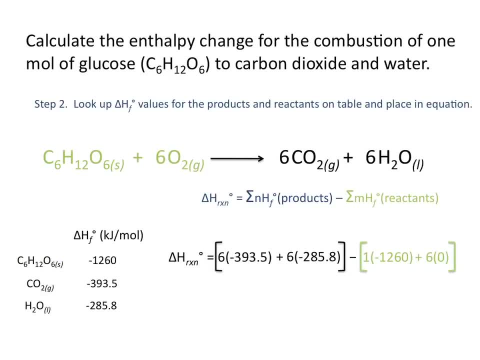 standard state is zero. these are the enthalpy of formation values for the reactants multiplied by their respective coefficients, and now it's a matter of correctly putting these values into your calculator to come up with the correct answer. be very careful, keeping track of your negative signs and the parentheses so you come up with 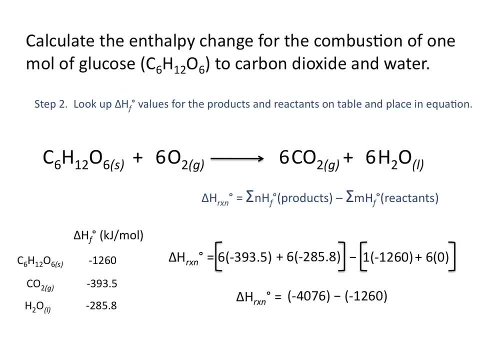 the right answers, and I think it's best to do these problems step by step, writing out the values you get for each part of the equation along the way. and this leaves me with an enthalpy value for the reaction of negative two thousand eight hundred sixteen kilojoules per mole. let's look at: 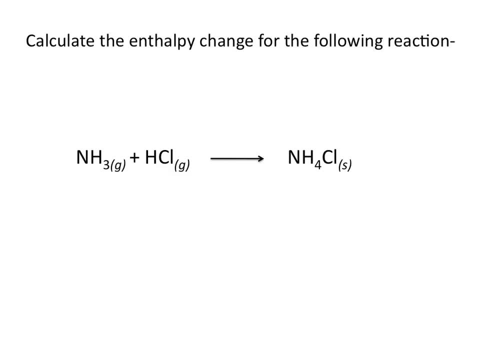 another example. calculate the enthalpy change for the following reaction: ammonia plus hydrochloric acid goes to ammonium chloride. the first step is to check that you have a balanced chemical equation, and in this case our equation is already balanced. the next step is to plug our enthalpy of formation values. 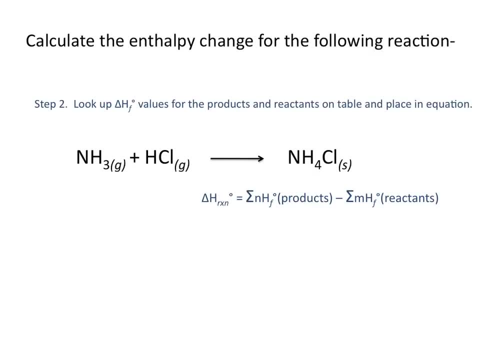 into our equation. so we look up the enthalpy of formation values for the products and reactants on the table. on the product side we have one mole of ammonium chloride and the Delta H of formation of ammonium chloride is negative three hundred fourteen point four kilojoules per mole. on the reactant side we have one mole of. 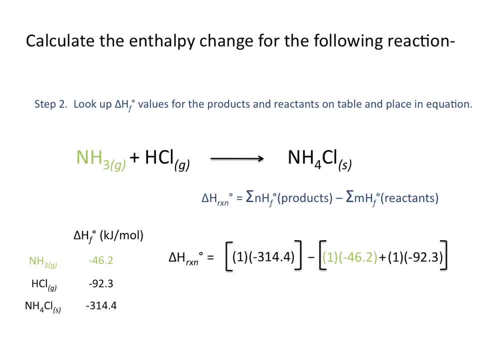 ammonia multiplied by the Delta H of formation value for ammonia negative forty six point two kilojoules per mole. and also one mole of HCl as a gas, which you multiply by its Delta H of formation value negative ninety two point three kilojoules per mole. we then take the sum of the values for the products multiplied.